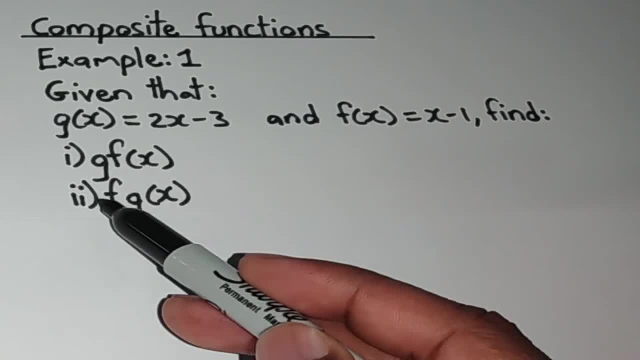 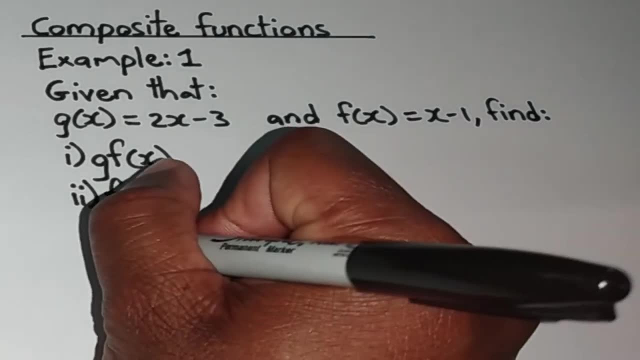 find part 1, g of f of x, part 2, f of g of x. alright, Now let's see how we can evaluate these types of questions. Let's start with part 1,. alright, So here we have g of f of x. 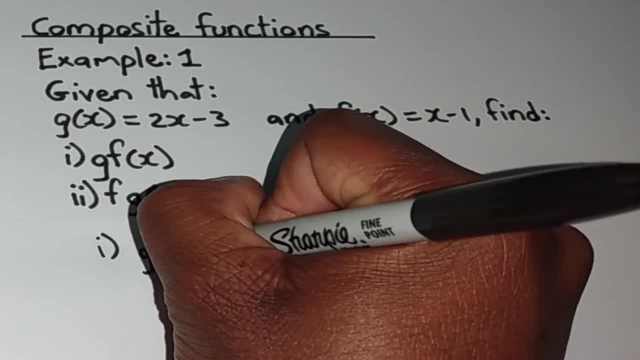 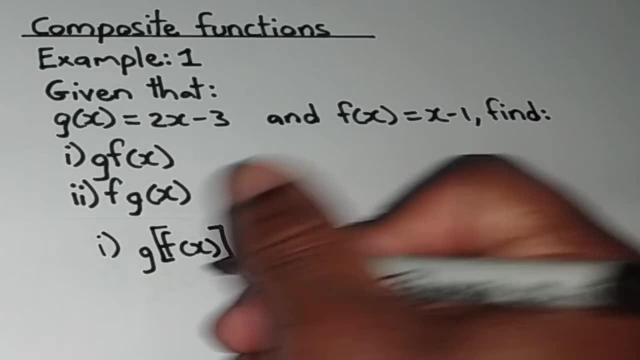 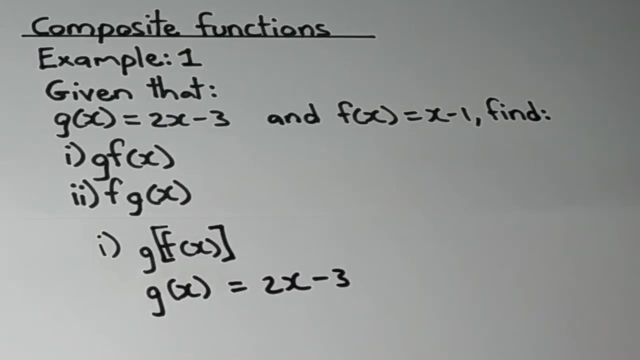 alright, And this is the same thing as substituting the entire f of x function into the g of x function. alright, So let's see how we can treat with this. Recall that the g of x function is equal to 2x minus 3, alright, So that's the g of x function, right there Now. 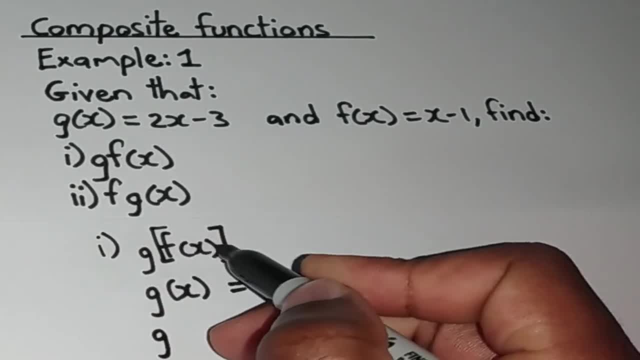 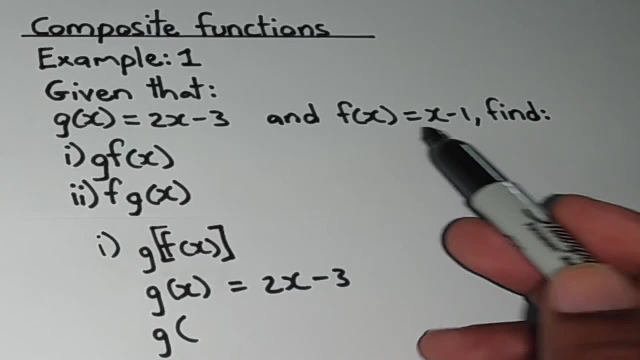 what we're going to do in order for us to find g of f of x, we're going to substitute the f of x function into the g of x function, alright, So, in other words, wherever we have x, we are going to replace the x with x minus 1, which is the f of x function. alright, So here we go. 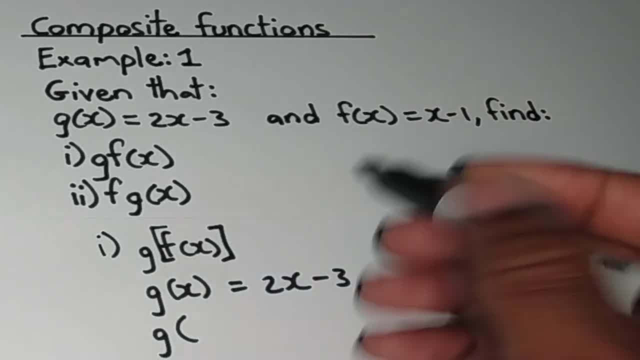 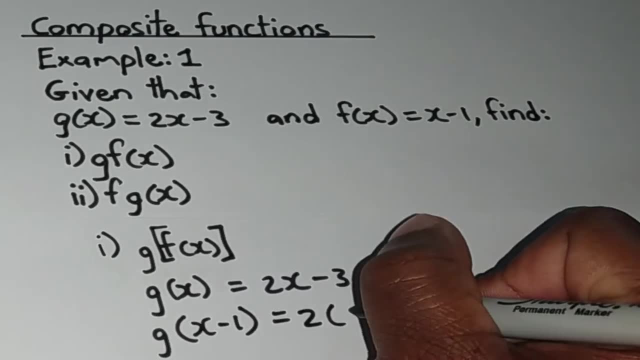 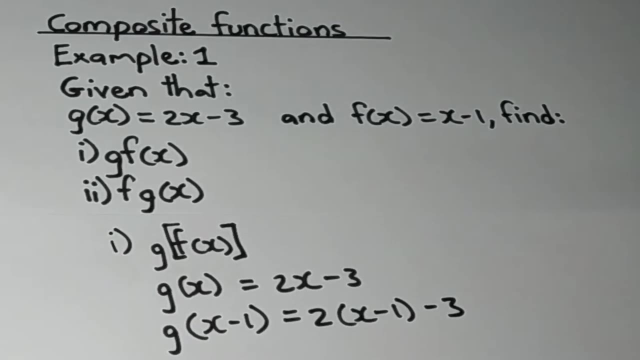 So right away, I'm going to replace this x here with the f of x function, which is x minus 1, alright, So wherever I have x, I'm going to replace the x with x minus 1, alright, And here I have the minus 3,, just the same, alright. Now, what we can do, I can use. 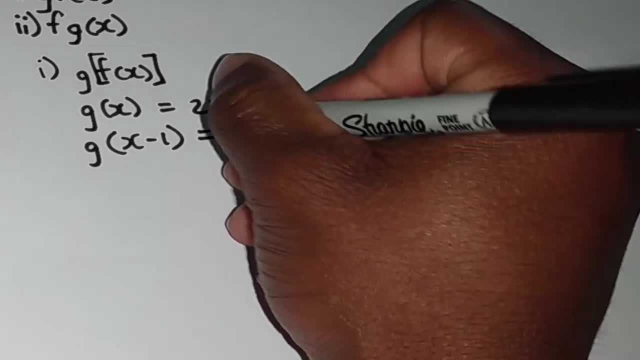 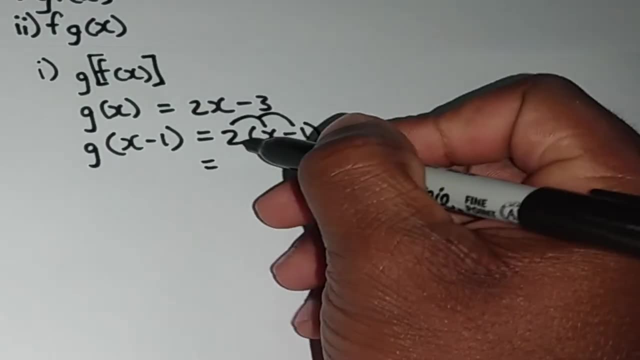 the distributive law to expand this bracket right here. So I can have 2 times x and 2 times negative 1 as well. alright, So I'm going to use the 2 to multiply each term in the bracket, So 2 times x. 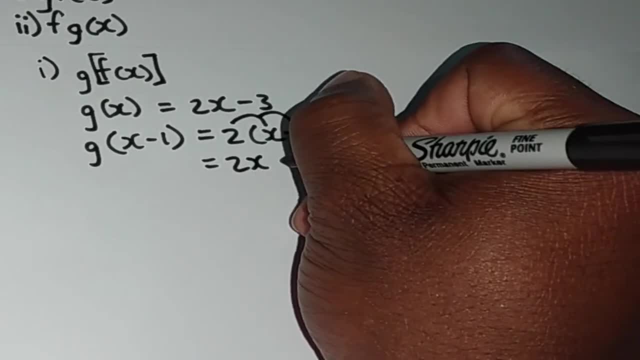 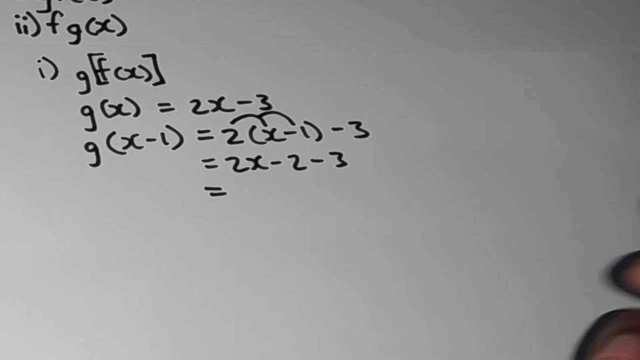 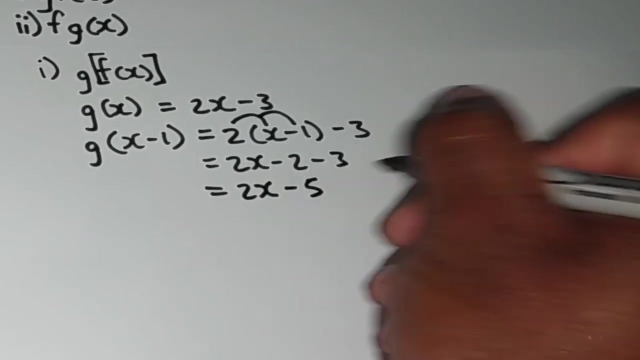 that will give me 2x, 2 times minus 1, that's negative 2, and I still have the minus 3 out here. all right, now we can simplify this thing some more, so we have the 2x. what's minus 2 minus 3, of course, that's minus 5, all right. so therefore G. 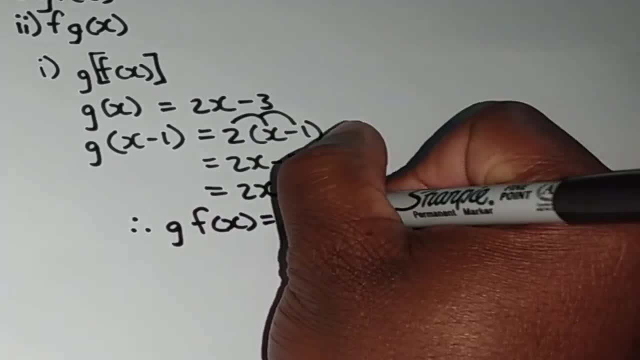 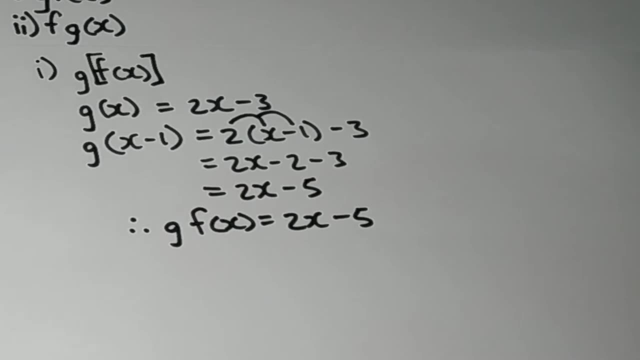 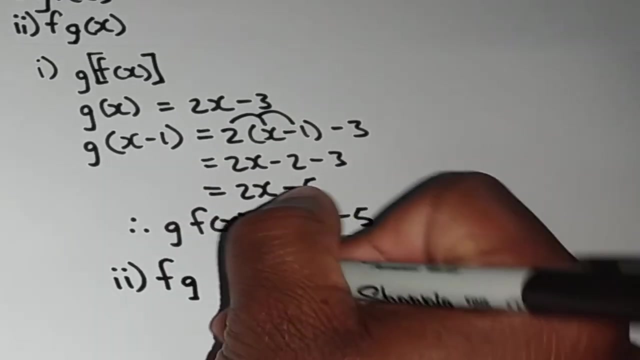 of f of X is equal to 2x minus 5. all right, so that's basically how we treat with a problem like that one in part 1. now let's see how we treat with part 2. all right, so now we are required to find f of G of X. all right, and this time, 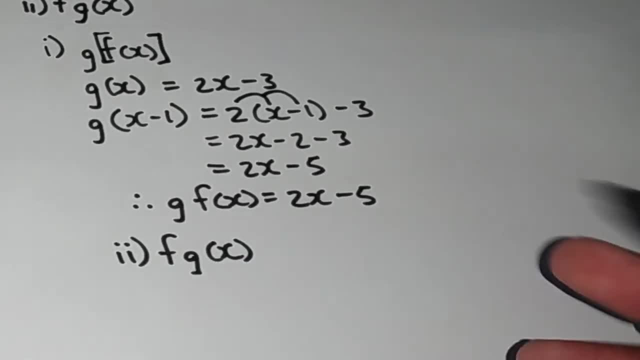 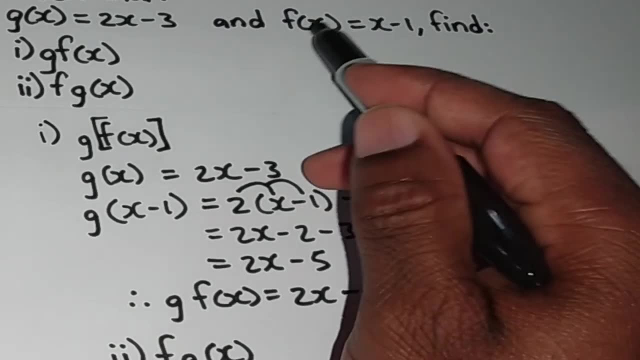 around. we are going to substitute the G of X function into the f of X function. all right, so first thing. first we want to recall the f of X function, which is this right here. so f of X is equal to X minus 1. all right, so we want to recall: 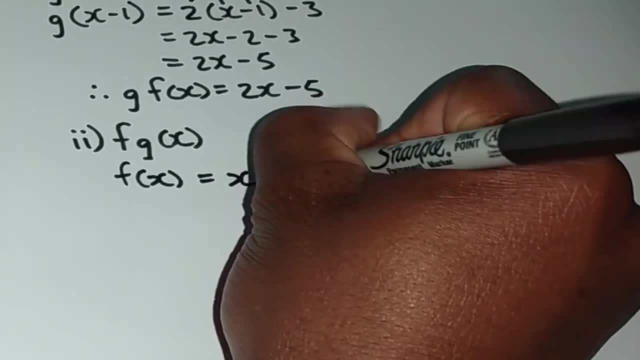 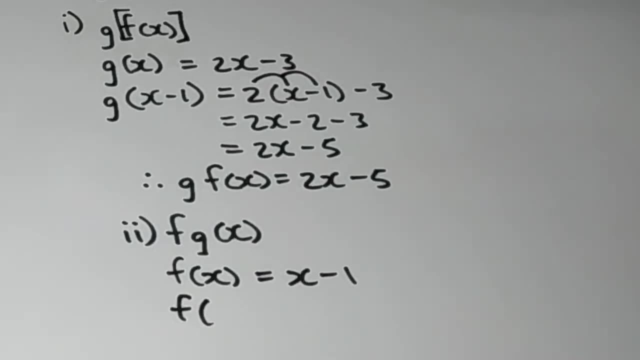 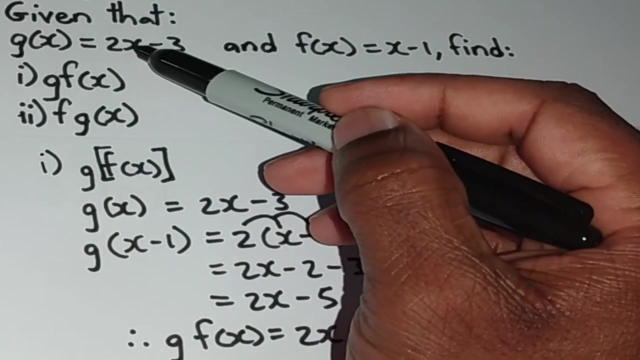 that. so f of X is equal to X minus 1. all right, so in order for us to find f of G of X, we're going to wherever we have X, we're going to replace the X with the entire G of X function. all right, so here we have G of X being equal to 2x minus 3. so we are. 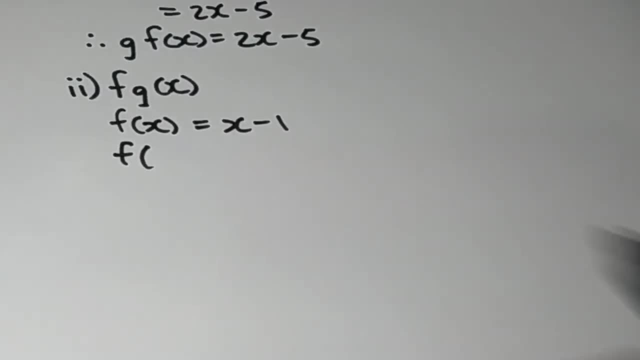 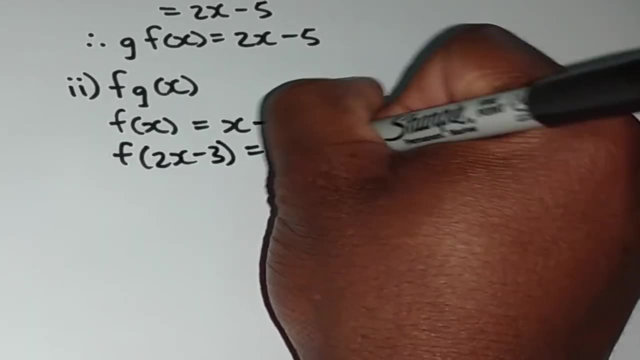 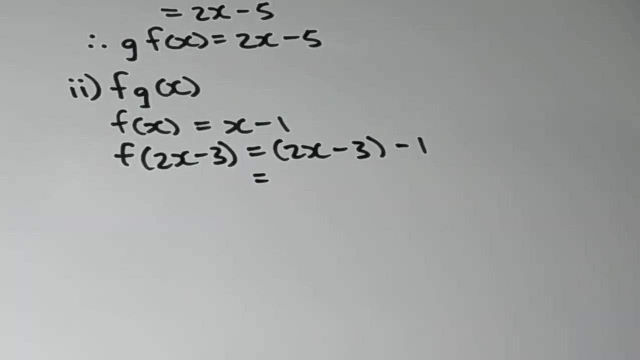 going to replace the X here with 2x minus 3. all right, so 2x minus 3, all right. so wherever we have X over here, we're going to replace the X with 2x, with 2x minus 3. I still have the minus 1 out here. now we can get rid of the. 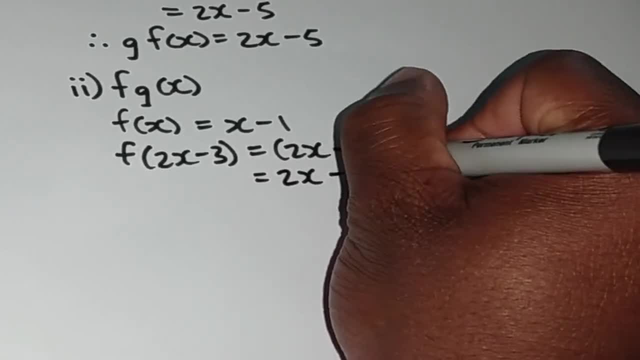 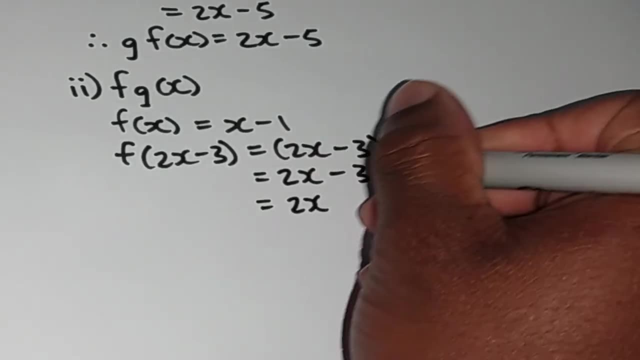 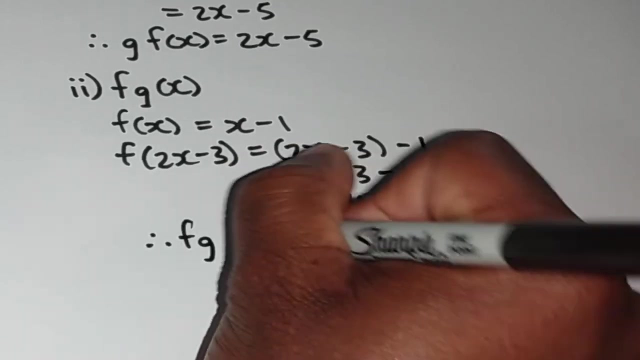 parentheses. so we are left with 2x minus 3 minus 1. we can always simplify this thing some more, so we're left with 2x minus 3 minus 1. of course that's minus 4. so we can say therefore: f of G, of X is equal to 2x minus 4. 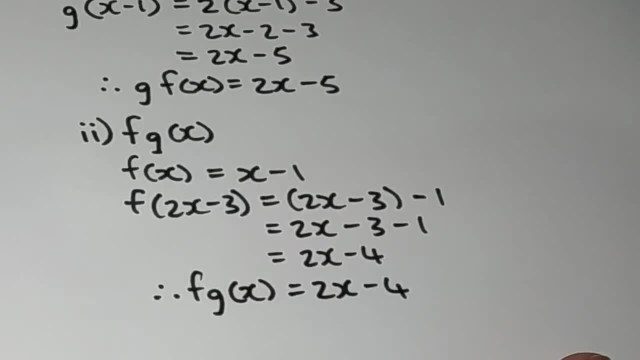 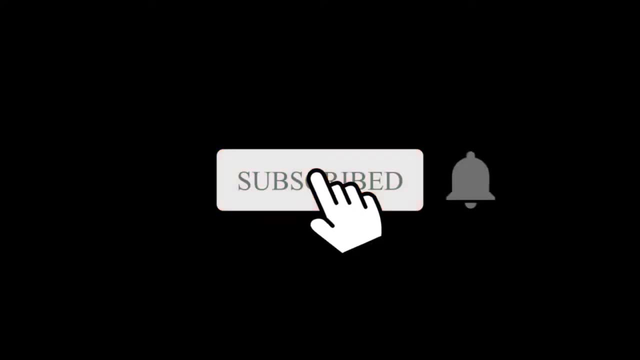 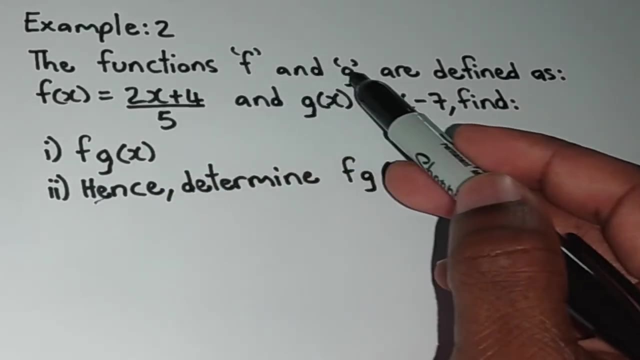 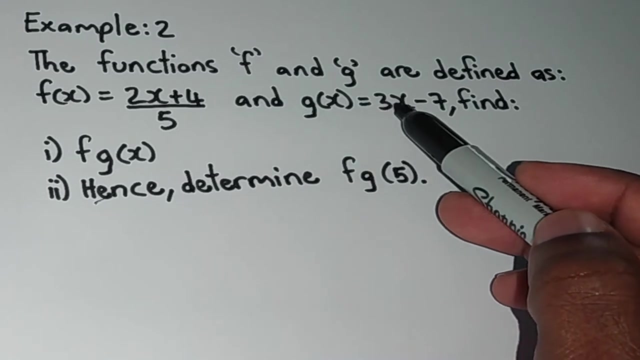 all right. so that's pretty much how we treat with the problems that we were given in example 1. all right, now let us look at example 2. now we're looking at example 2. all right, so the functions f and G are defined as: f of X is equal to 2x plus 4 all over 5, and G of X is equal to 3x minus 7 all. 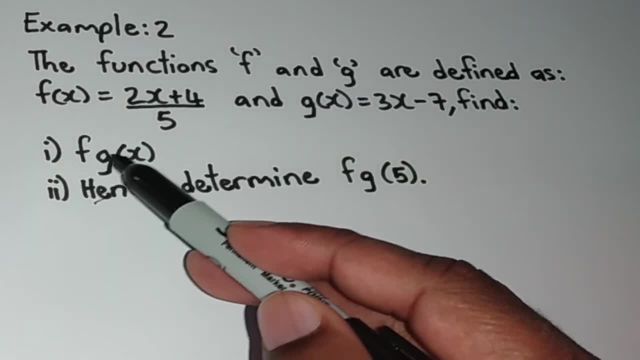 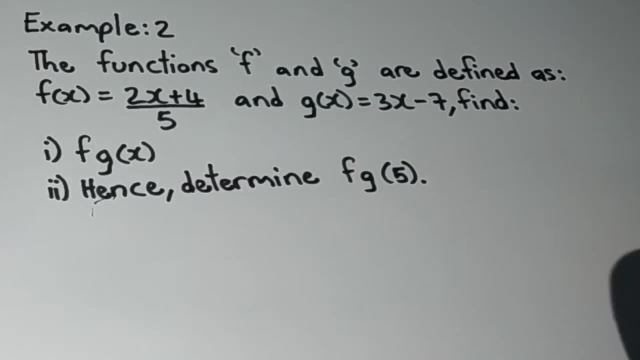 right, and from this they ask us to find part 1, f of G of X, part 2, hence determined f of G of 5. all right, and once we see the word hence here, then we know that part 1 is related to part 2. now let's see how. 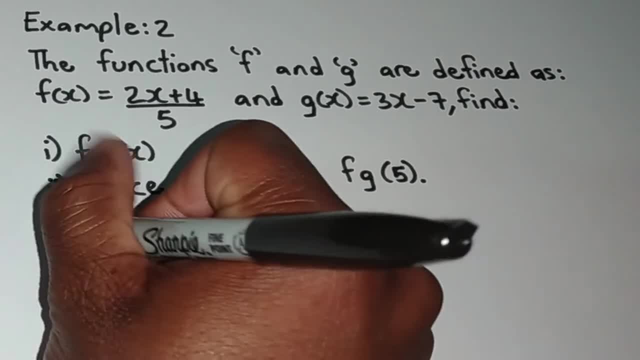 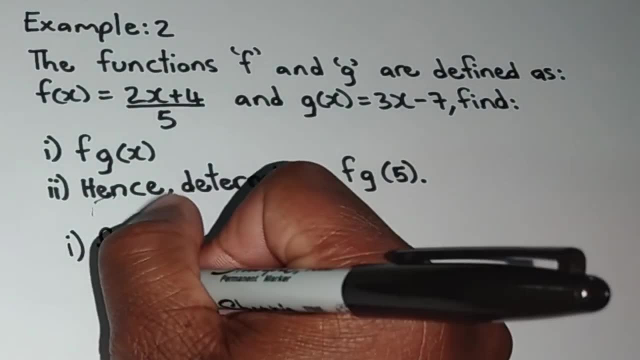 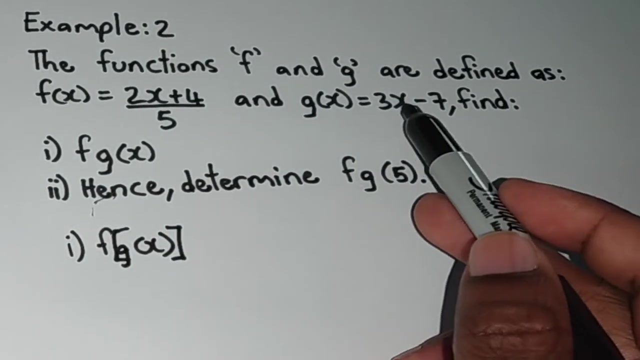 we treat with a question like this one. all right, so here we have part 1, and we want to find f of G of X. all right, and again, just like example 1, if we want to find f of G of X, then that simply means we're going to substitute the G of X. 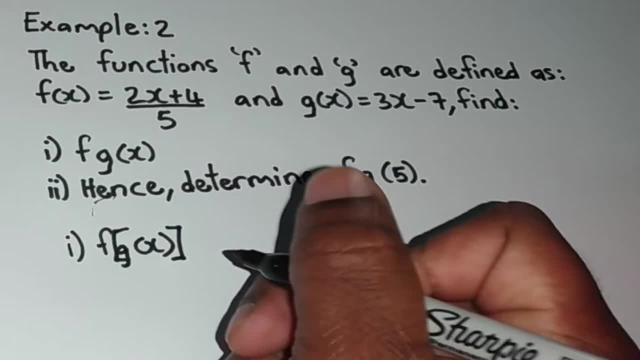 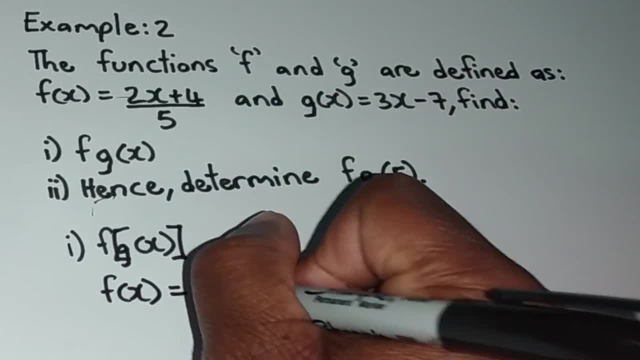 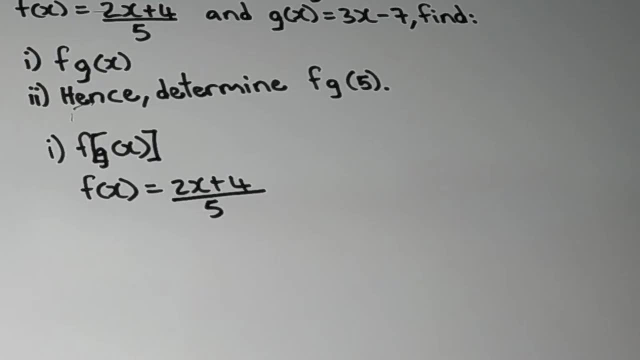 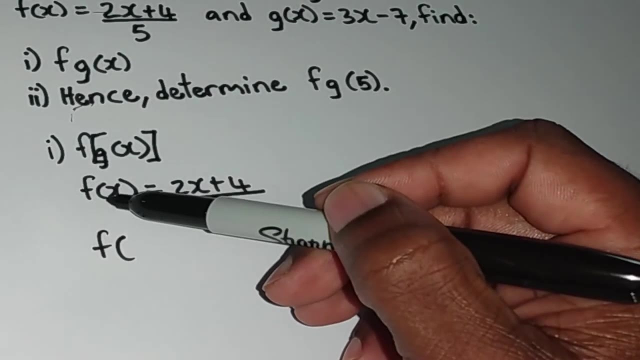 all right, which is this thing right here. so f of x is equal to 2x plus 4, all over 5. all right, and what we want to do now is to substitute the g of x function into the f of x function. all right, so wherever we have x, we're going to replace the x with the 3x minus 7. all right, so replacing the 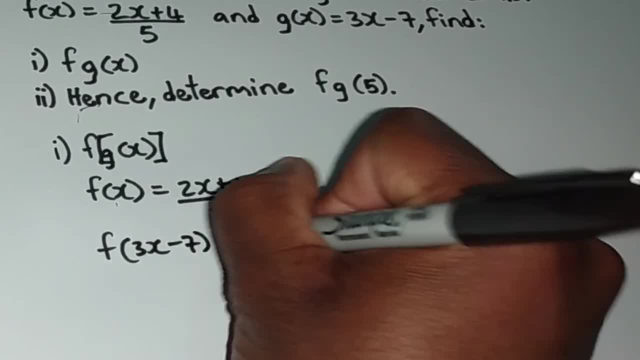 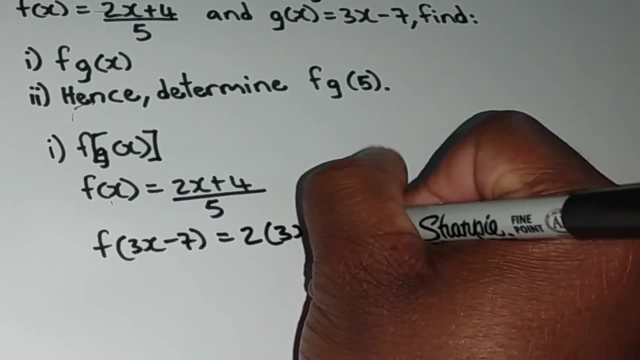 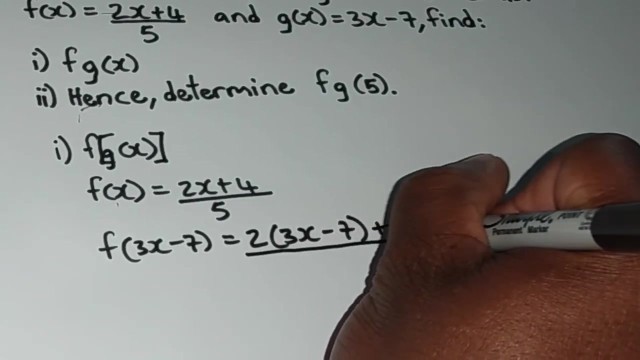 x here with 3x minus 7, all right. so wherever we see x in this function, we're going to replace the x with 3x minus 7, right? 3x minus 7. still have the positive 4 here all over 5. all right now. 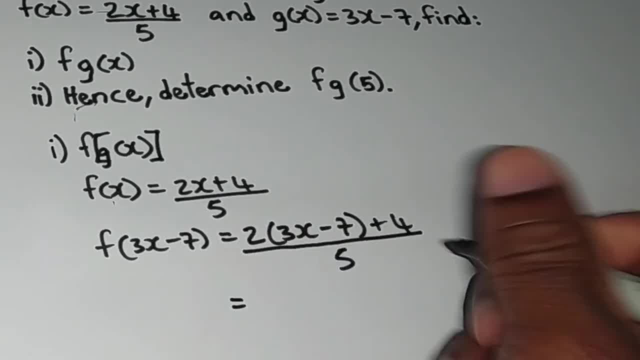 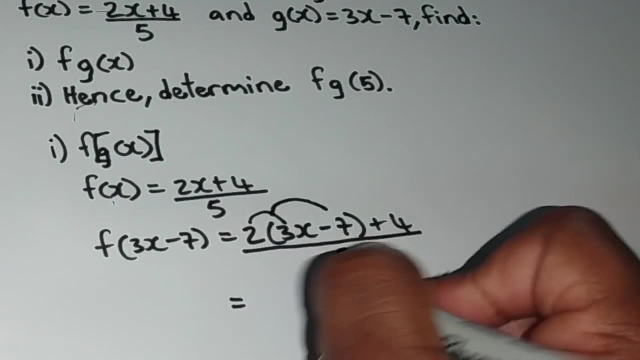 we can always simplify. all right, so, using the distributive law, we're going to use this tool here to multiply each term inside the bracket. all right, so using the distributive law, we're going to use this tool here to multiply each term inside the bracket. so 2 times 3x, that's 6x. 2 times negative: 7, that's negative 14. still have the positive 4 out here. 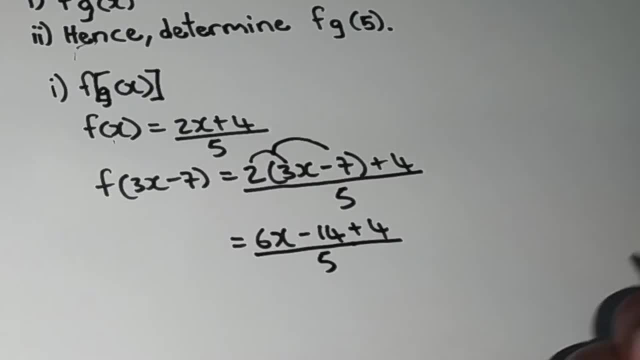 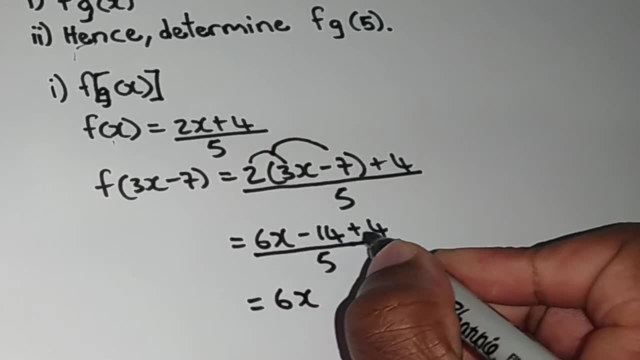 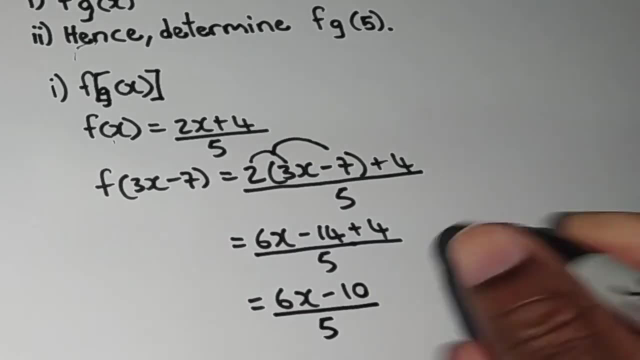 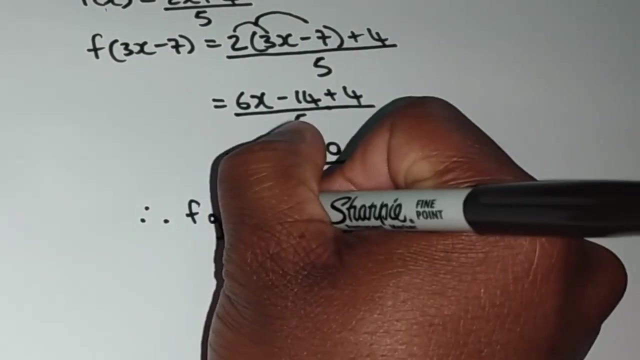 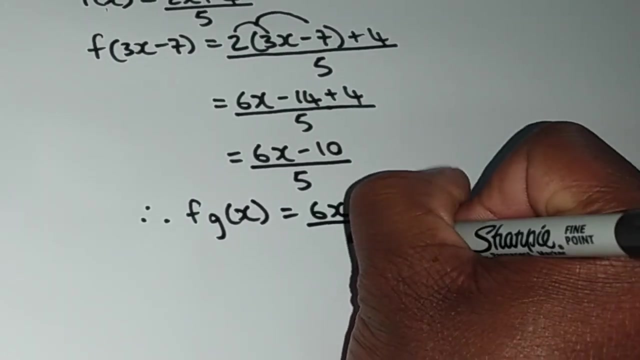 and this is all over 5, all right. now we can simplify some more. so we have 6x, what's negative? 14 plus 4. of course this is negative 10, all right, and this is all over 5, all right. so therefore we can say: f of g of x is equal to 6x minus 10, all over 5, all right. so this is our f of g of x function. 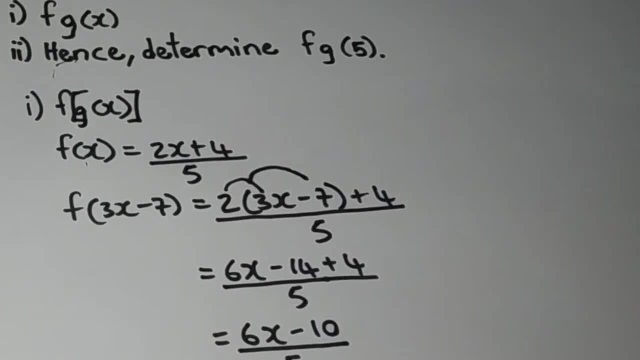 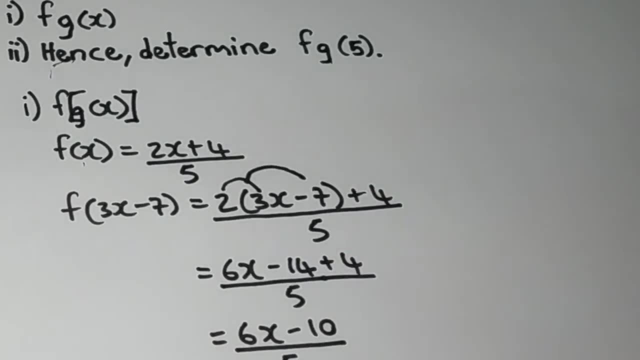 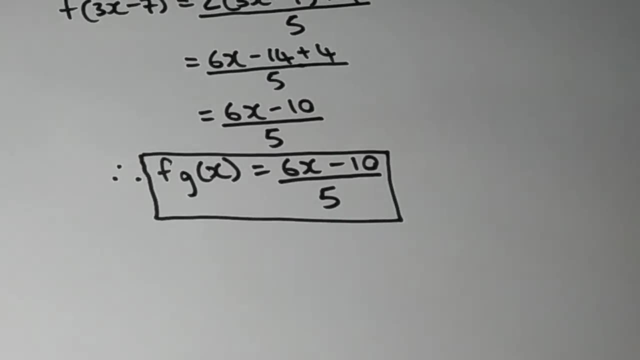 all right. now let us see how we treat with part 2, all right, which is hence determine f of g of 5. all right, and before we can find f of g of a given value, then we first must know that f of g of x function which we just found all right. so what we can now do is to simply substitute. 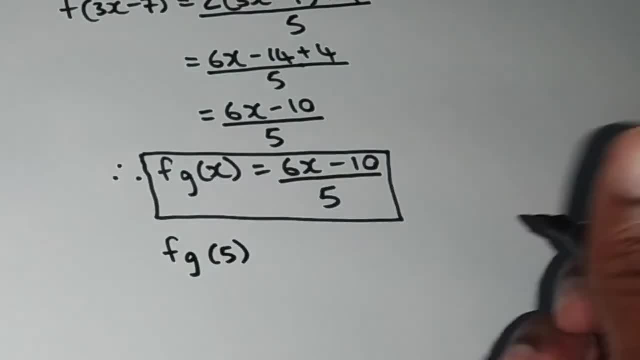 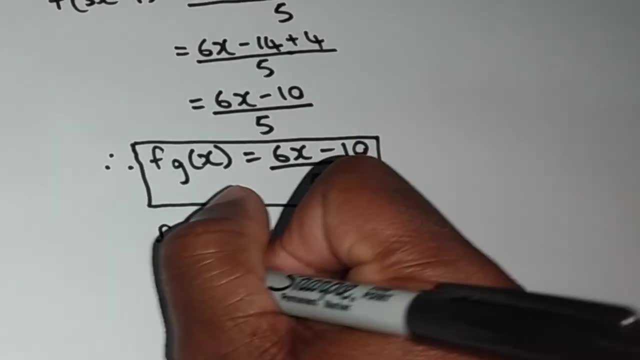 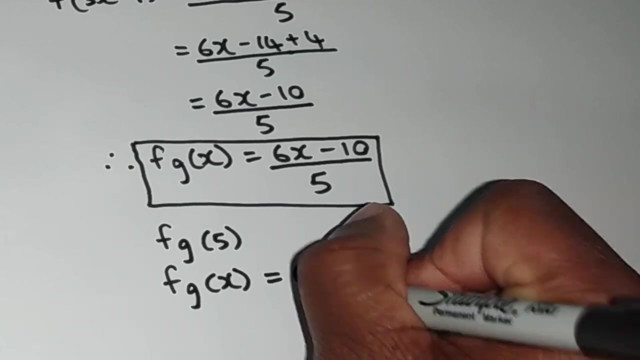 the value of 5 wherever we have x in the f of g of x function. all right. so this is the f of g of x function here. so f of g of x, we know is equal to 6x minus 10 all over 5. all right. so if we want to,